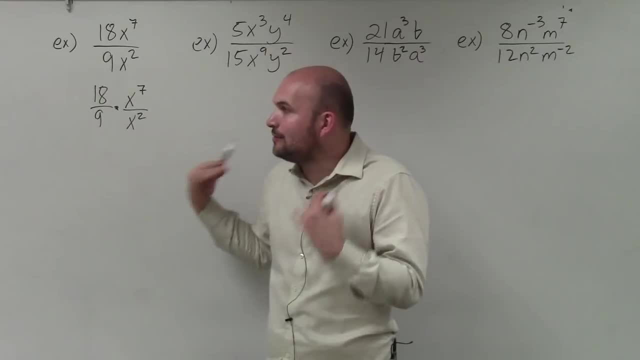 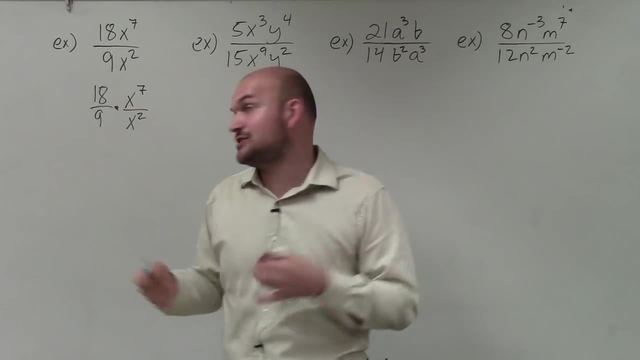 And the reason why I like to do this is because then it kind of helps me separate the numbers and the variables. So in the numbers, what I'm simply doing is just simplifying this fraction. I have 18 divided by 9, which is really meaning how many times does? 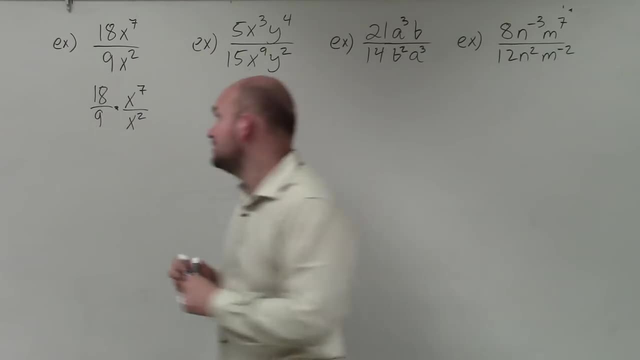 this divide 9 going to 18.. Well, I can just simplify that to 2.. For the case of rational expressions, though, we're going to write 2 as 2 over 1, so that we know that the 2 is in the numerator. 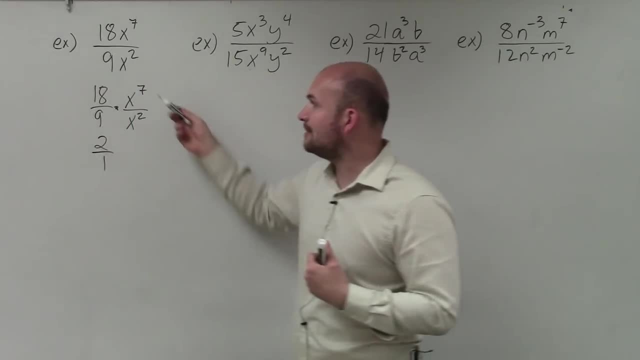 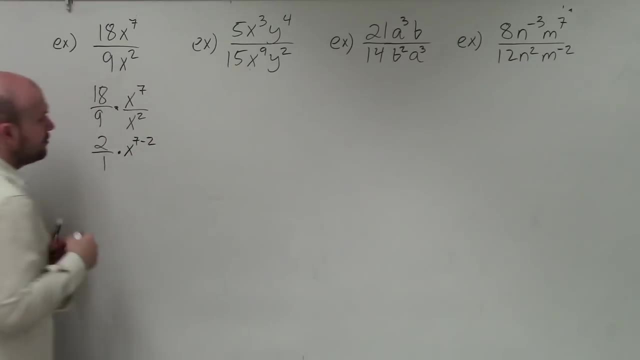 and the 1 is in the denominator. Now, by using the rules of exponents, I have x to the 7th over x squared. So I'm going to use the quotient property, which is going to tell me to do x to the 7th minus 2.. So I'm going to be subtracting them, which is going to leave me with 2, 2. 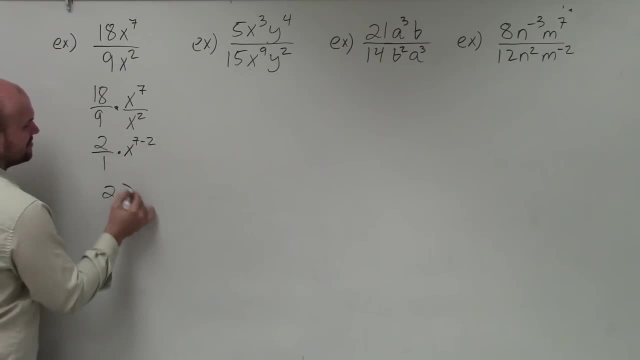 over 1,, which is, and x to the 7th minus 2, is going to leave me with x to the 5th. Now, those are both going to be in the numerator, So therefore we don't really need to rewrite. 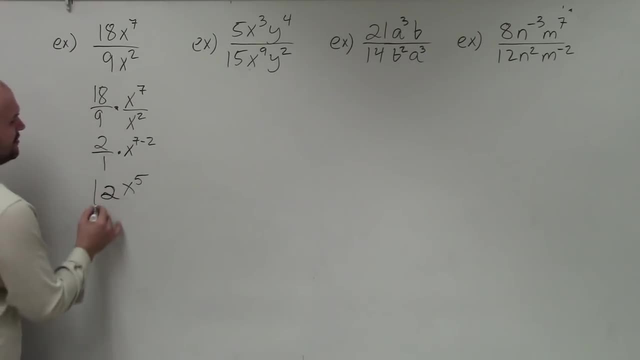 them over 1.. So I'll just rewrite my finalized answer as 2x to the 5th. Now let's go over in this example And, as you can see over here, you got those. Now you can go and see in this example: now I have x's and I have y's, But you're going. 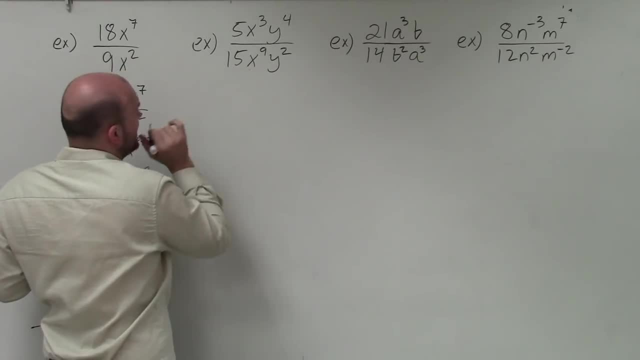 to apply the same operation. You don't have to break them apart in this case, But I kind of like to again, as we're getting started with. this is to break them apart. so I know which rules of exponents I have: x's and y's. 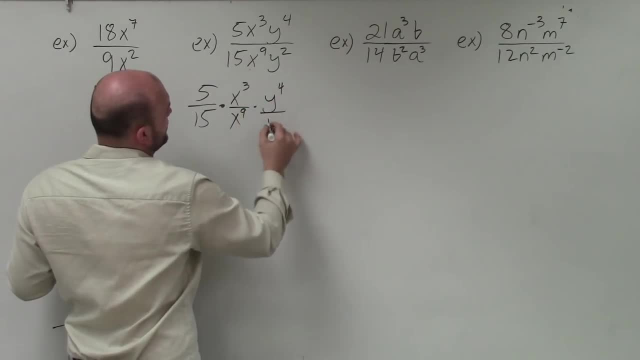 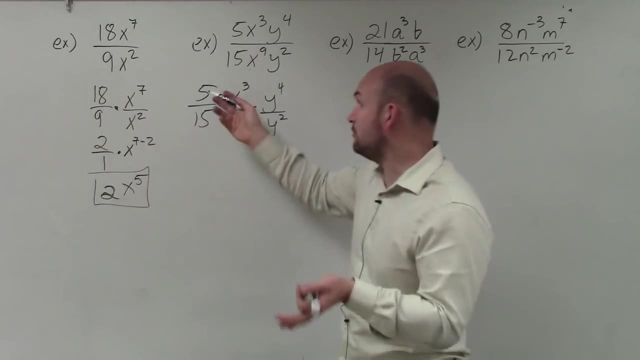 Exponents. I am going to apply here. So I have y to the 4th over y squared Now again. now, in this case, this is what trips up a lot of students is they see over here, oh, 9 goes into 15.. And they say, oh well, 5 goes into 15.. But remember that's. 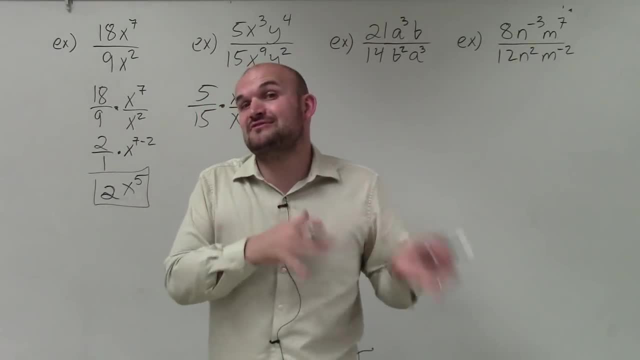 not what this one is saying. It's saying 5 divided by 15.. Or how many times does 15 go into 5?? Well, 15 is larger than 5, so it doesn't evenly divide. So what we're going to do is: 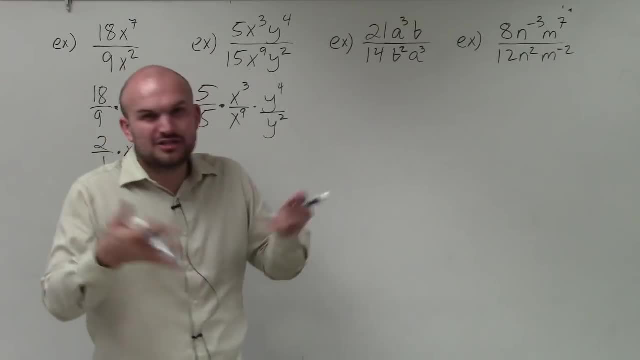 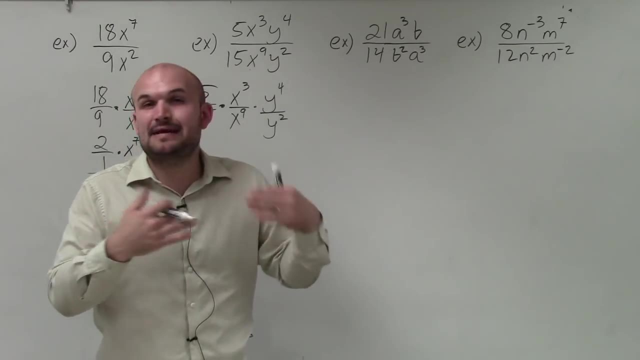 we're going to have to simplify this, And by simplifying basically what we're doing, just like I say, you know, 4 halves is the same thing as what It's. I'm sorry, 2 fourths is the same thing as 1 half, And the reason why we can do that. 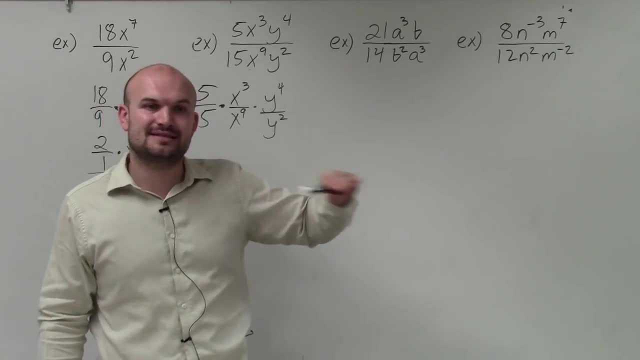 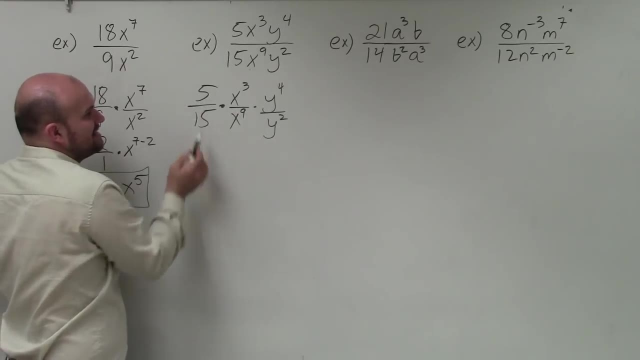 is, as long as we divide the same number in the numerator and the denominator, we are keeping an equivalent fraction. So I look at this fraction and since 15 doesn't divide into 5, I say: all right, well, is there a number that divides evenly into the numerator? 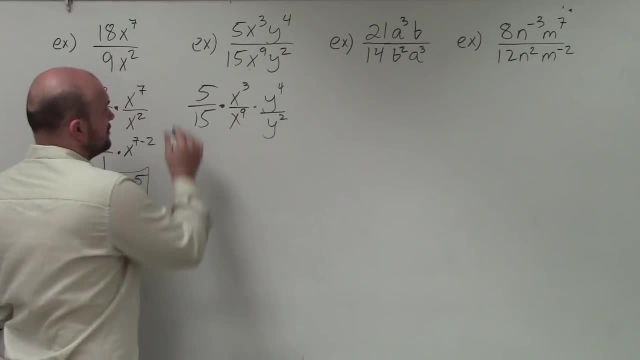 and the denominator, And that number in this case is 5.. So if I divide the top by 5, I get 1.. If I divide the denominator by 5, I get 3.. So 5 15ths can be reduced down to 1. 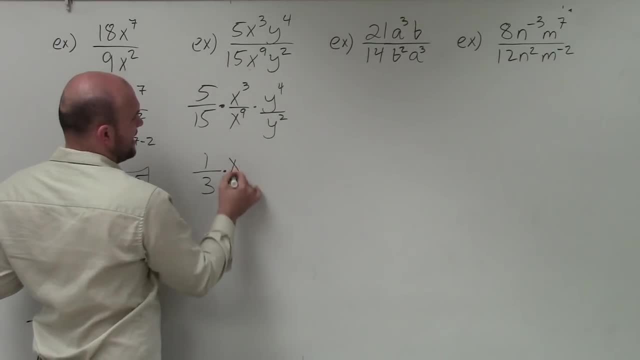 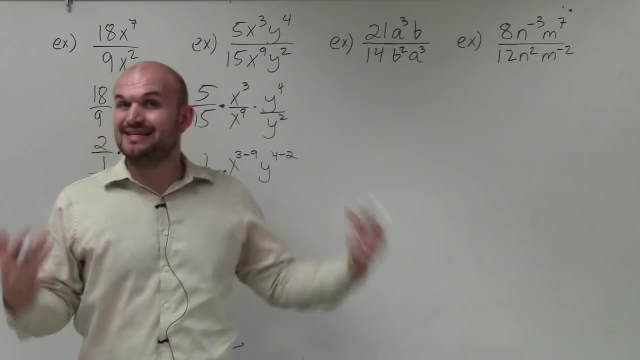 third: Now I apply the rules of exponents over here. So I have x to the 3 minus 9.. And here I have y to the 4th minus 2.. Now, if you remember, in my video on rules of exponents with negative, 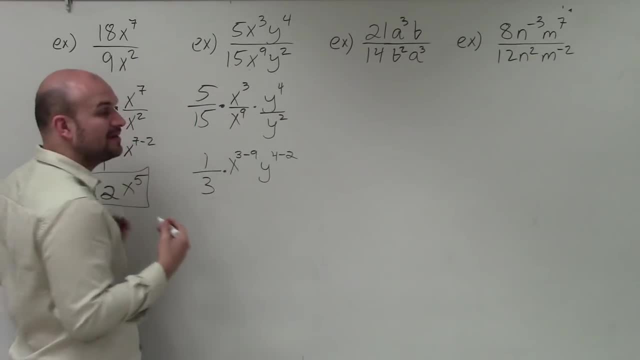 exponents. it's very important to understand that. how to rewrite a negative exponent in your negative exponent as a positive. So I have 1 third times. now these are going to be in the numerator when we write them. So that's going to be x to the negative, 6.. 3. 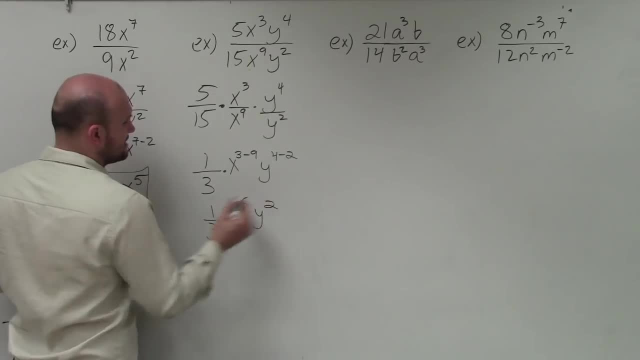 minus 9 is negative 6. And this is going to be y to the 4th minus 2.. So that's going to be y to the 2nd And, as I remembered when dealing with negative exponents, to rewrite: 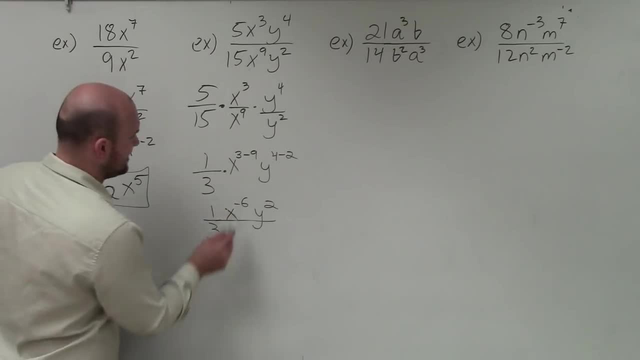 a negative exponent as a positive, we're going to rewrite it as its reciprocal. So my final answer would be: 1 times y squared, which is just y squared, all over 3 times. now x to the positive 6th power. Again, that's going to be dealing with your y. This is in the 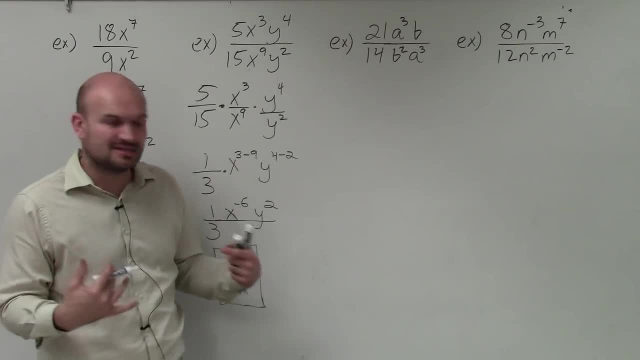 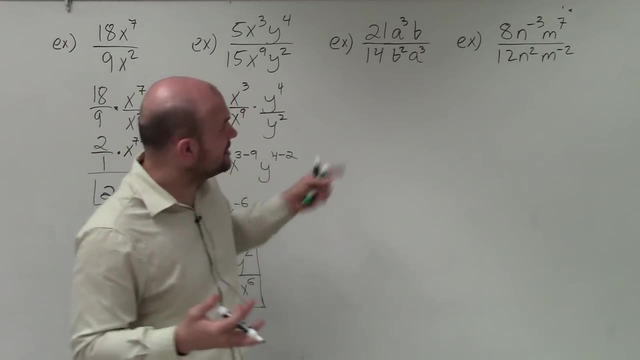 denominator Again goes through my rules of negative exponents. So if you have more questions on that, please make sure you go back to that video, just to make sure you have a full understanding. Now, in this case this one gets a little bit trickier because you can see now the a's and 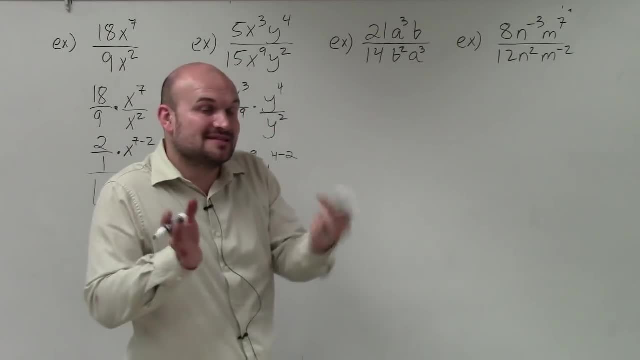 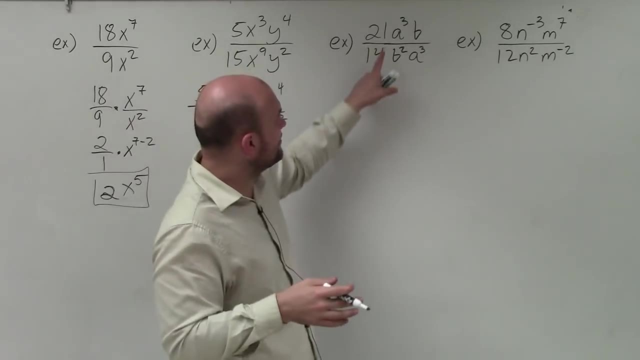 the b's are not aligned. Well, fear not, We can just simply align them. Since it's multiplication, we can just rearrange them any way we want to. Just like 2 times 4 is the same as 4 times 2, we can just rearrange b squared times a cubed as a cubed times b squared. So I'm just 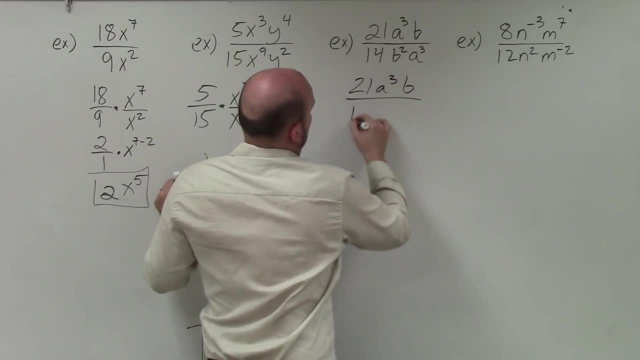 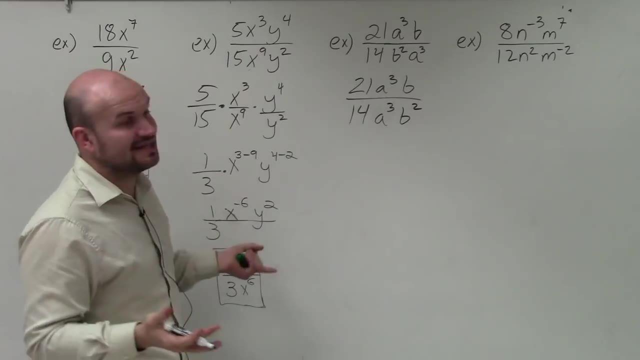 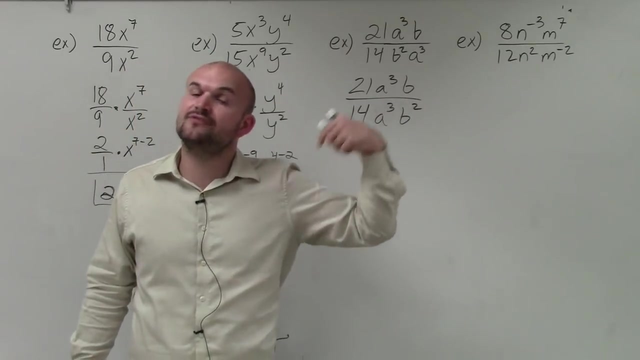 going to rewrite it. Got to rewrite those. Switch them right. OK, So now, in this case again, we are going to simplify this. Now. in this case, though, 14 does not evenly divide into 21. So I want to look to see if well, can I reduce these? Is there a number that? 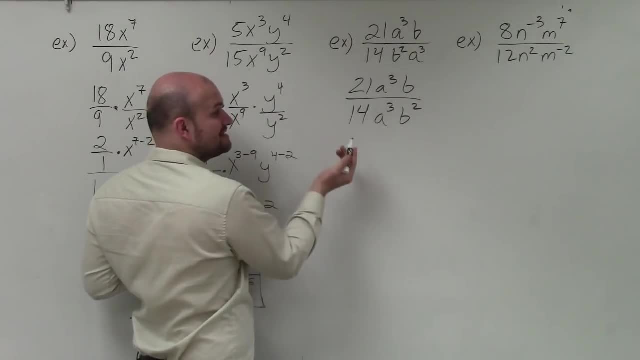 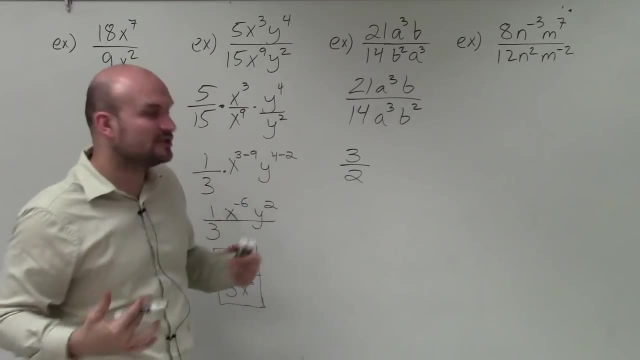 divides into both of them- And, yes, a number that divides into both of them is 7.. 7 divides into 21, three times, and 7 divides into 14, 2. So 21 over 14 can be reduced to 3 halves. 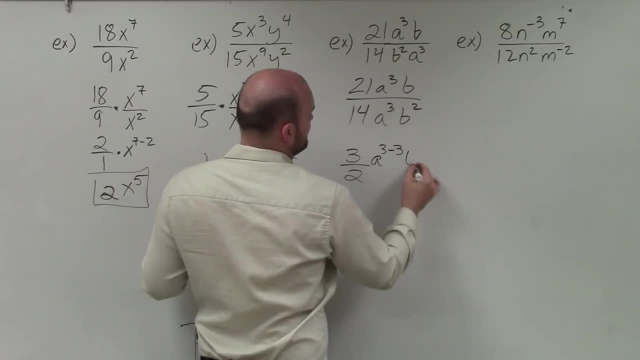 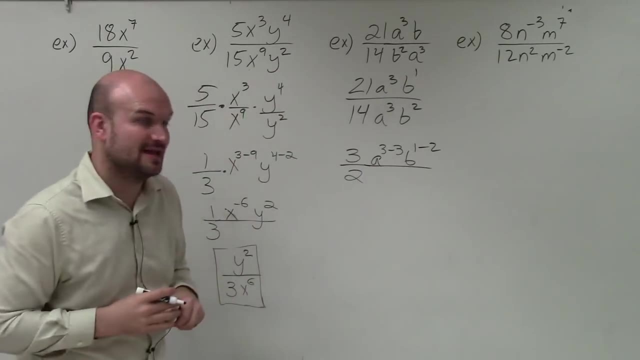 Now, over here, I have a to the 3 minus 3 and b to the 1, because there's a 1 up there, if we don't have anything listed- minus 2.. Again, those are all written as in your numerator. So then I have 3 halves. Well, a to the 3. 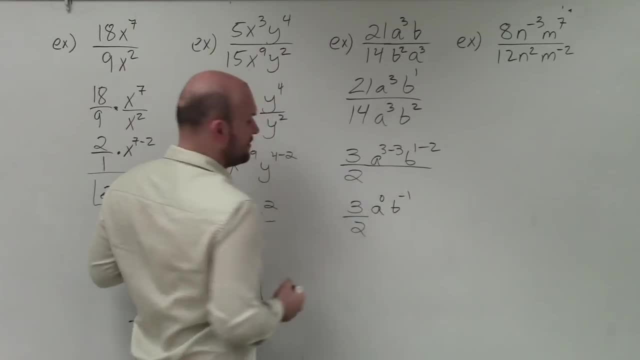 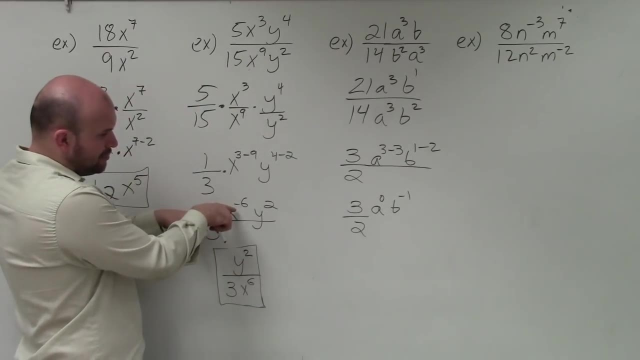 minus 3 is going to be a to the 0 power and then b to the negative first. Now remember: anything raised to the 0 power is just going to be 1. And b to the negative first, just like we had over here: if it's negative in the numerator, to rewrite it as positive. 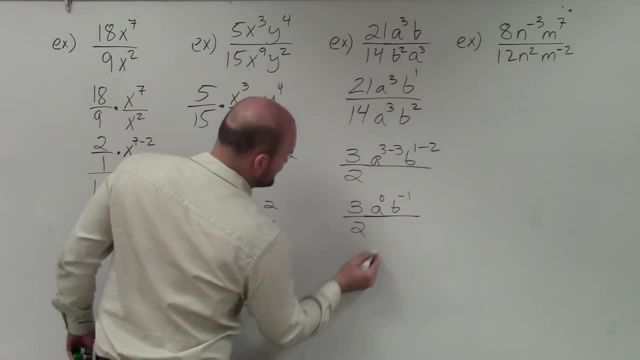 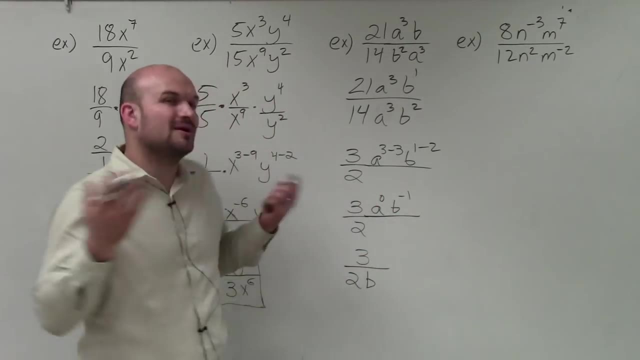 we're going to need to put it in the denominator. So therefore, my final answer is going to be 3 times 1, which is a to 0.. So that's just going to be 3 over 2. b to the first power. 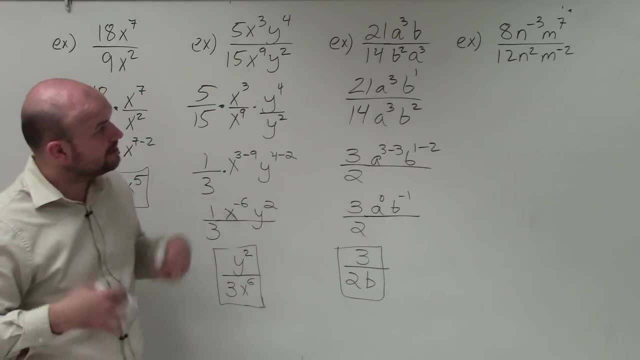 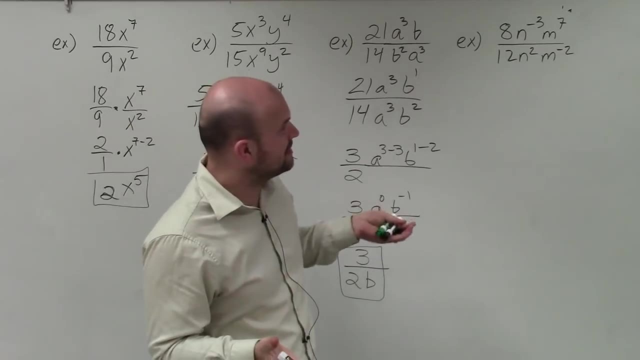 So that's going to be 1 up there, So we'll just leave it as 3 over 2 b. And then my last example. you can see I have negative exponents already. So there's a couple different ways you can do this. We can automatically make our exponents positive by putting this: 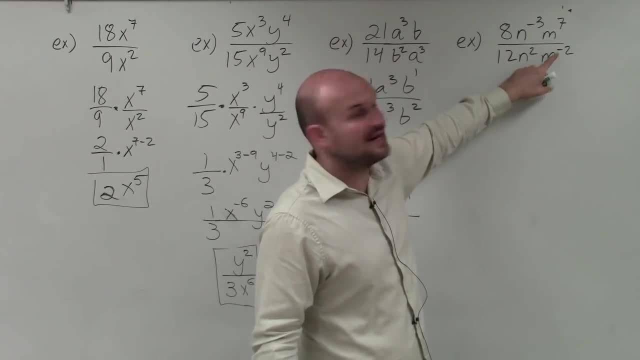 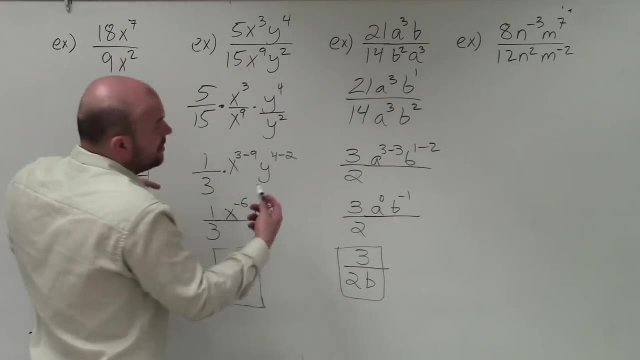 n to the negative, 3 down in the denominator and the m to the negative, second back in the numerator, Or we can simply just apply the quotient property already with them being negative. Now, I don't like dealing with negative numbers, So the first thing I'm going to do 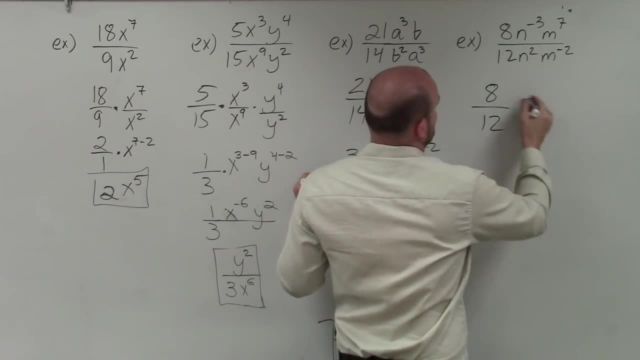 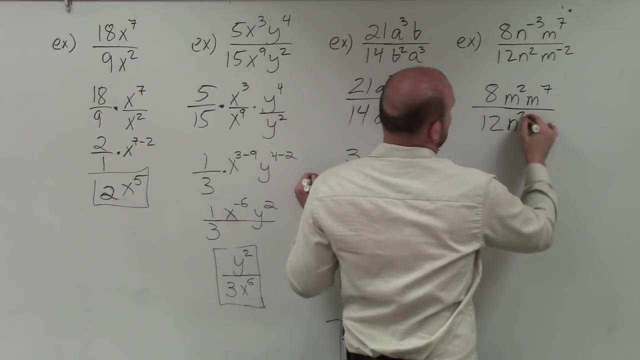 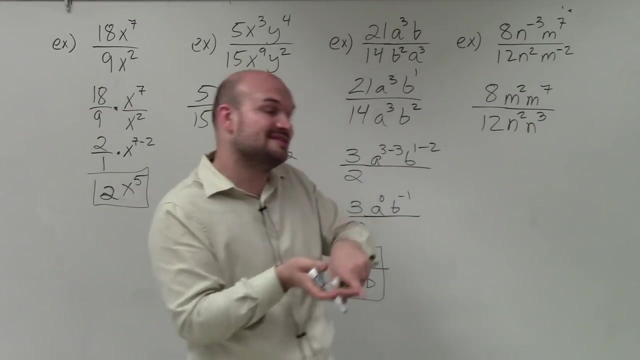 is rewrite them so they are all positive. So I'll have m squared times m to the seventh all over n squared times n cubed. Remember to make my negative exponents positive. I just put them in as the reciprocal. So if they're in the denominator negative I put 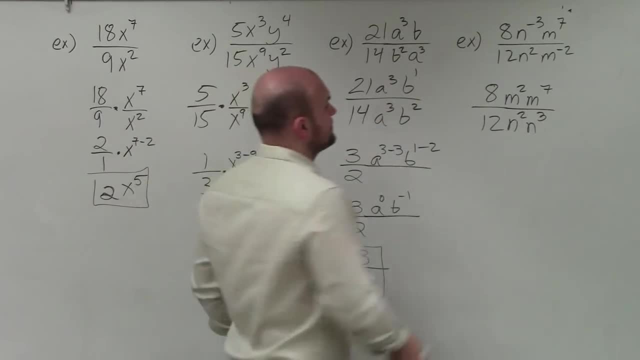 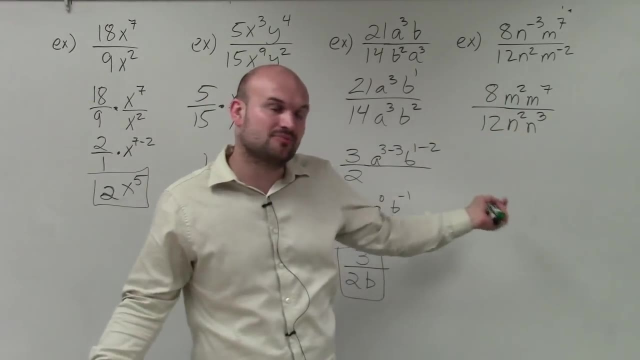 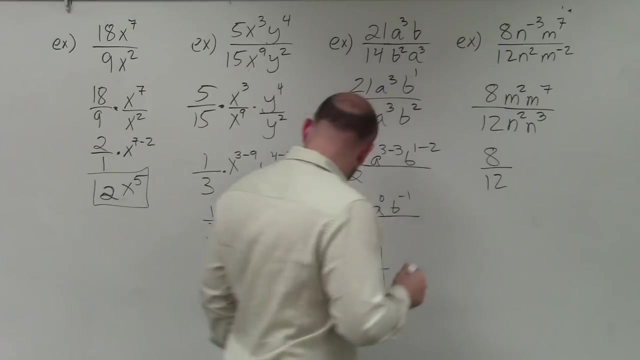 them in the numerator. If they're in the numerator negative, I put them in the denominator. Now I can't use the quotient property because the same bases are not in the numerator and denominator, So I'm going to use the product property. So with the product property states, oops. 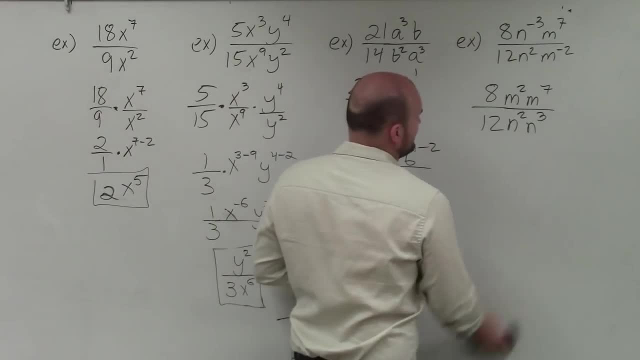 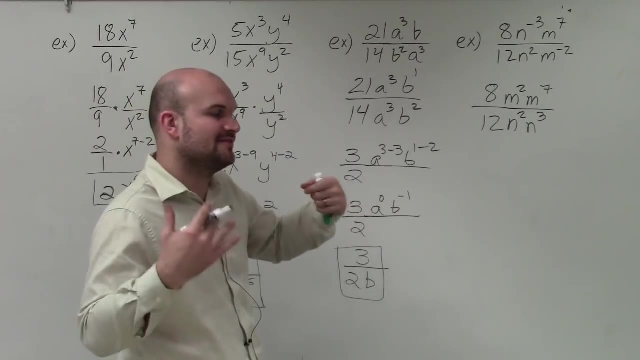 before I even get ahead of myself, let's go ahead and simplify 8 twelfths Again. in this example, ladies and gentlemen, 12 does not go into 8.. However, we can reduce 8 twelfths. So we want to think of a number that divides evenly into 8 as well as in 12. And that number 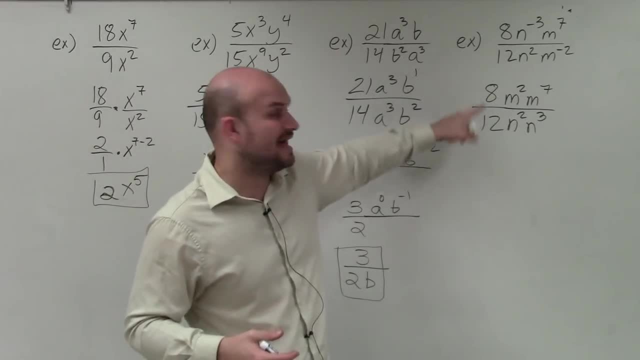 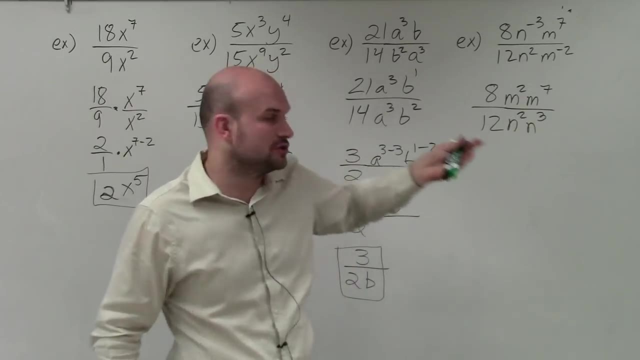 the largest number is going to be 4.. Even though 2 does divide into 8 and 12, if we divide by 2, we'd have 4 sixths, which could be reduced further Again by dividing by 2.. So you always want to choose your largest number, which is 4.. 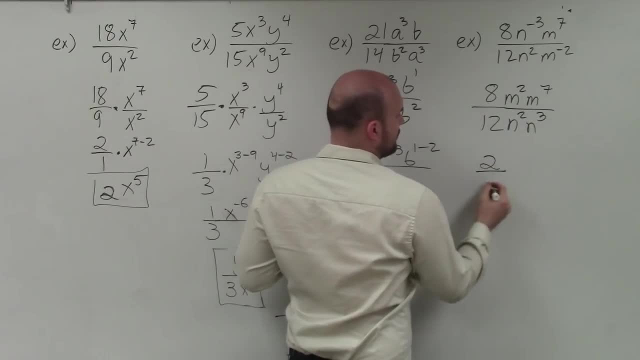 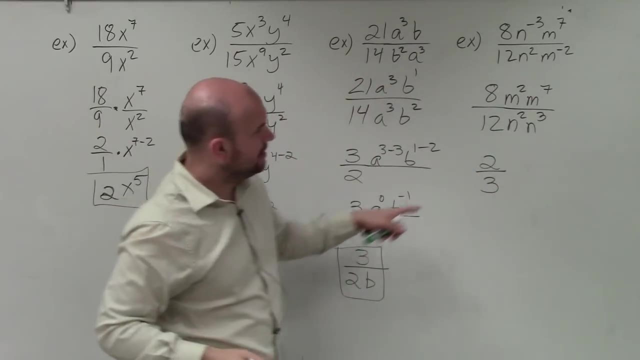 So if I divide 8 by 4, I get 2.. If I do 12 divided by 4, I get 3.. So therefore, 8 twelfths is reduced to 2 thirds. Now I can't use the quotient property like I did before, because 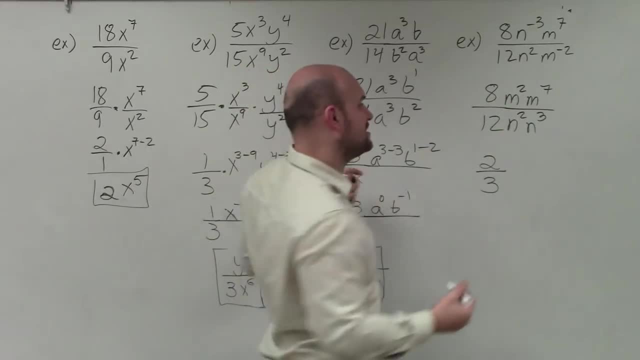 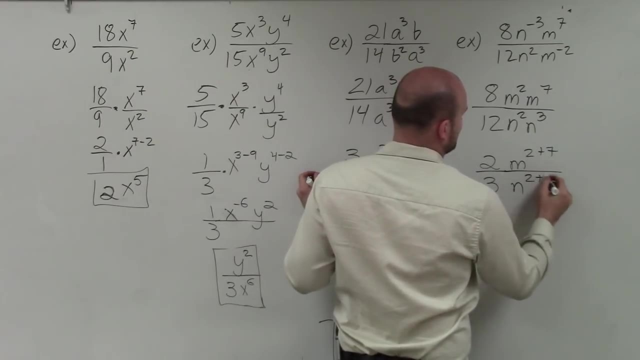 I don't have m and m's in the numerator and denominator, So I'm going to apply the product property which tells me to. when I multiply two exponents with the same base, I am going to add their powers. Okay, So now I have 2 to the nth. 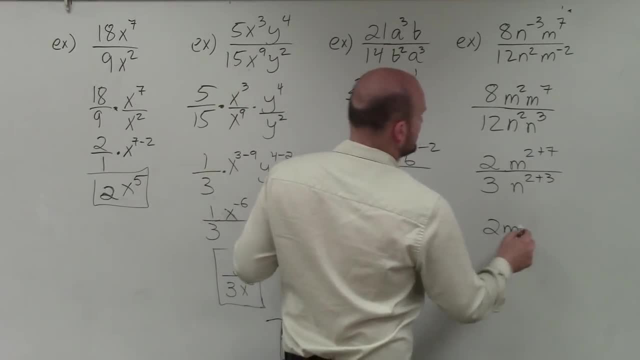 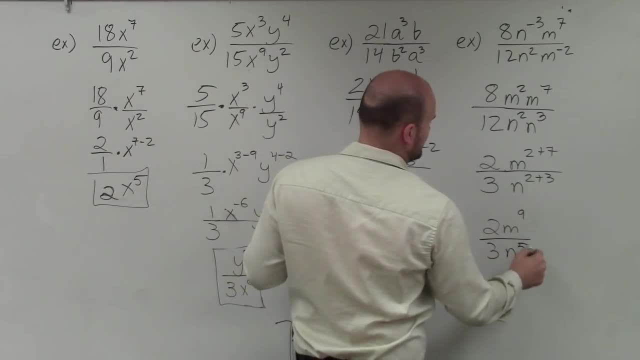 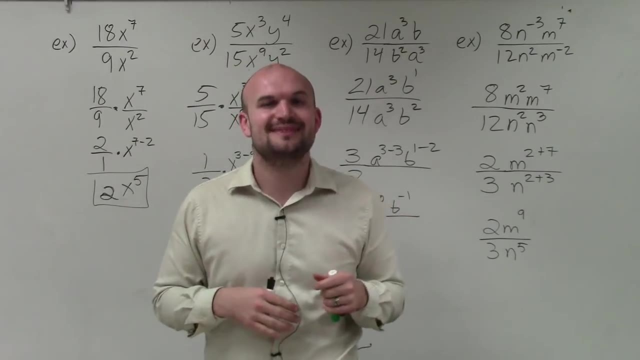 All over: 3 to the 2 plus 3 is going to be n to the fifth. So there you go. ladies and gentlemen. That is just your basic little overview of simplifying rational expressions by applying the rules of exponents. Thanks,